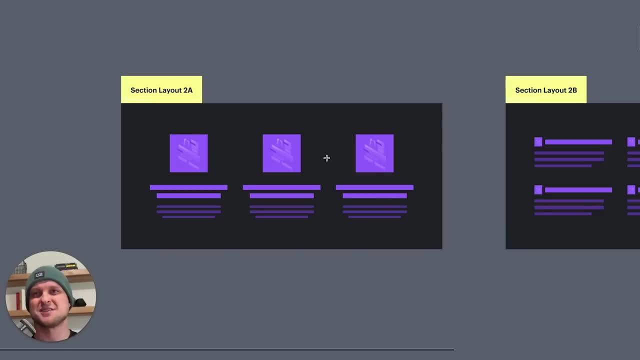 lay out your two, three, four most essential points with an image or an icon. You can have them in these three columns. Sometimes I'll see people use four columns, but if you do this you really have to shrink things down, But this layout is a great way to do that. So we're going to go ahead and we're going to 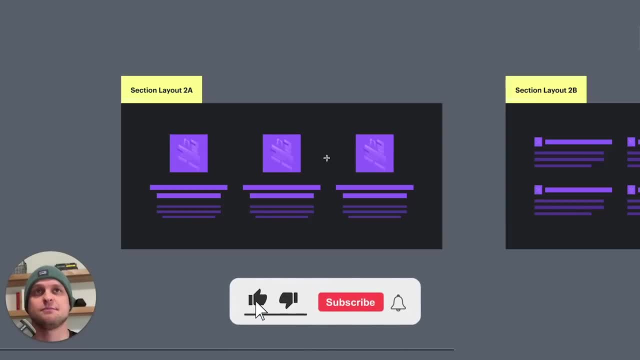 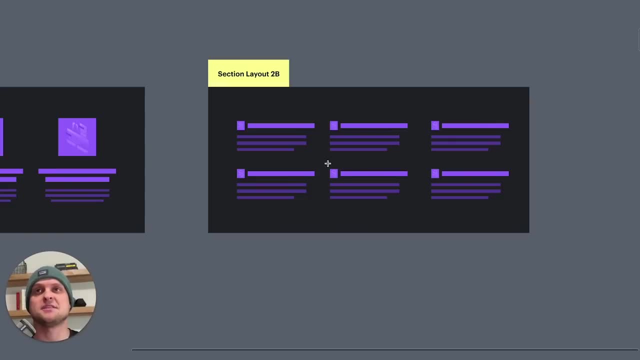 this more into like a grid where we've got an additional row and you can see that you can mix up the way you're using that image or the icon, just to make sure that it doesn't feel so basic and so much like a template. I do see oftentimes where people will have nine points. They'll have. 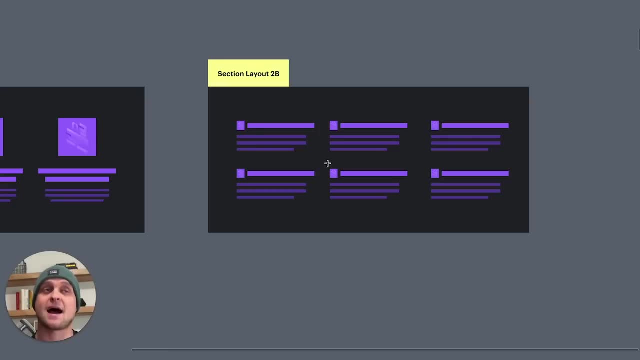 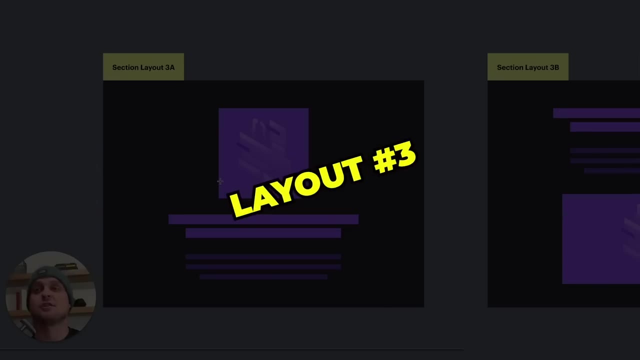 a three by three grid. I would never go more than this, And I even personally feel like six is kind of pushing it, So just keep that in mind, All right. So, moving down to section three, this is just a basic vertical centered layout, And 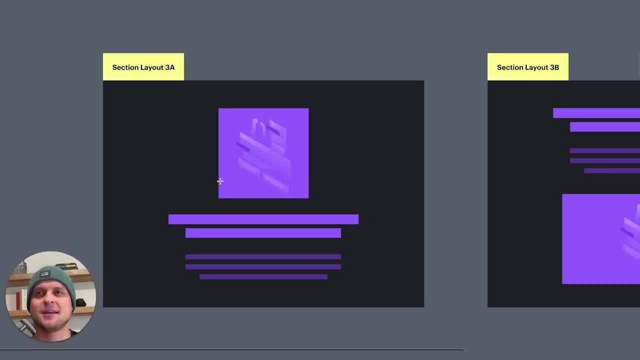 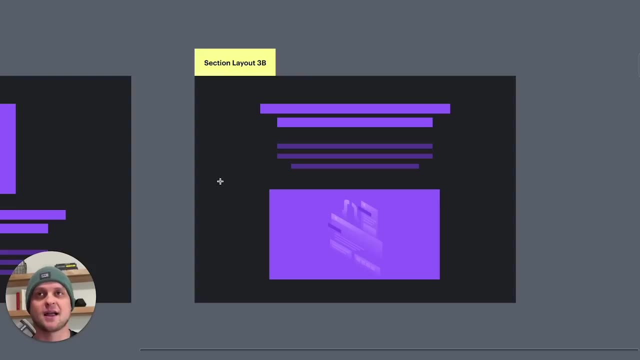 you're going to see this a lot, especially in like sales pages, landing pages, And you can see in a variation you really can put the image and the text and any different variation that you would like, But at the end of the day these are all going to be very similar because it's just the 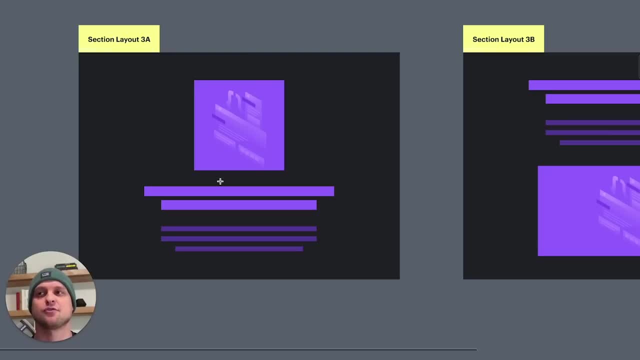 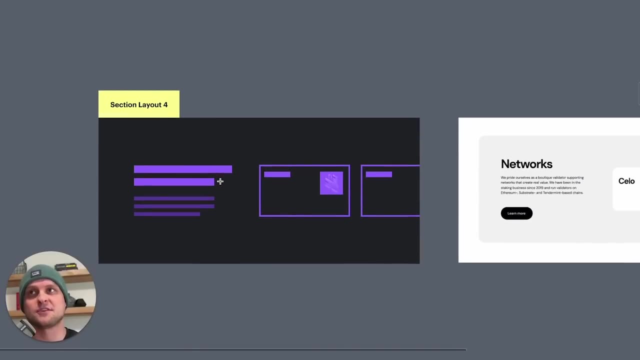 centered, aligned look. So section layout three is a great option. All right, So now we're going to get into a little bit more unique. Now, this first one that I want to share with you. this is section layout number four, And this is a really cool way to utilize a slider in a very small section. So 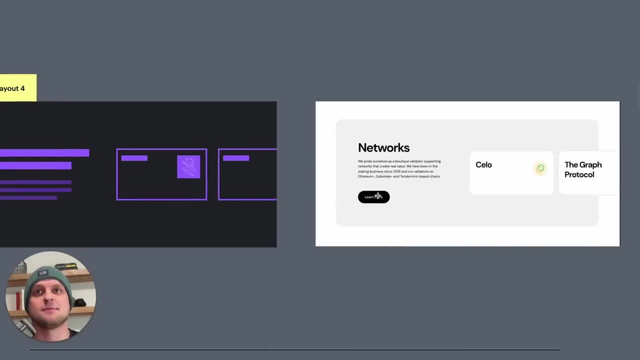 you can see here in the example, we've got our header, our subtext and our call to action here on the left, And then we've got a couple elements that are built into a slider, And you can see that we are illustrating the fact that it's a slider because one of the elements is trailing. 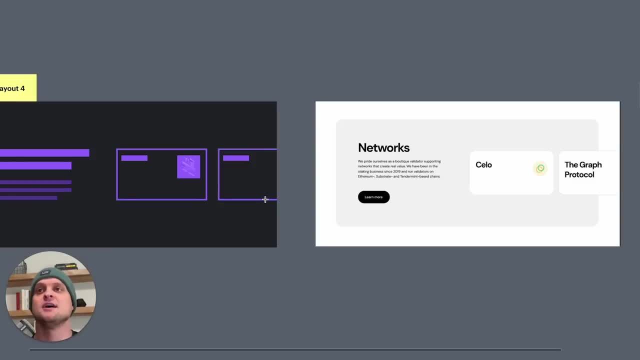 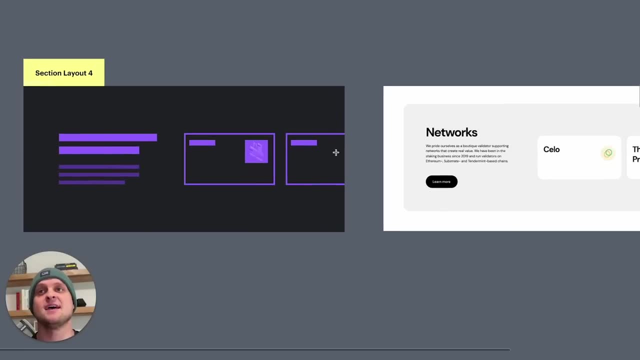 off the page And that says to me: okay, there's more to see, So there should be some way to slide and see those additional elements. Now, the one thing that we want to be aware of is if this slider slides and we don't do something to make this element on the left. 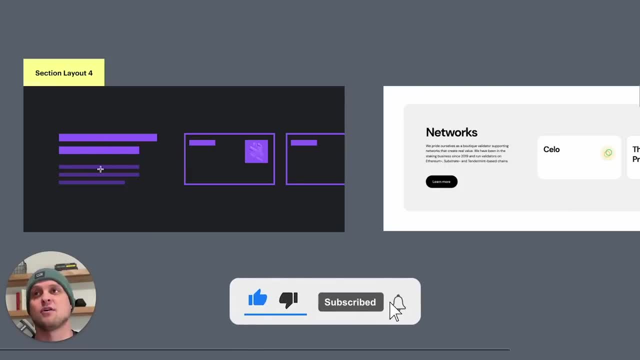 disappear, that's going to bump right into the things we have on the left or, even worse, is going to go right over the top of it. So we need to have some sort of opacity or something set here in the interaction, where it makes the left one disappear as the right one comes in. 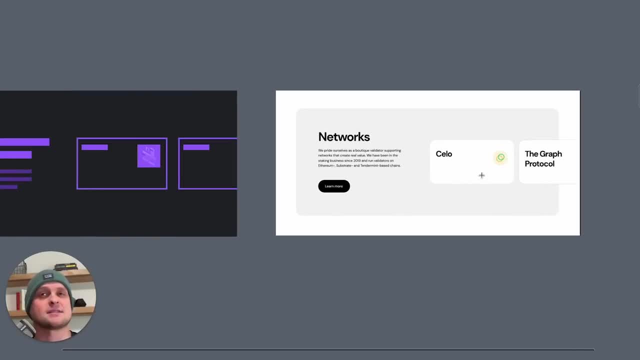 The other thing that we want to have is, unless this is set on a timer and it's moving pretty frequently, or if there is something where you can have like a pointer, a unique pointer, that they can click and drag, people aren't going to know what to do because there's not any sort of 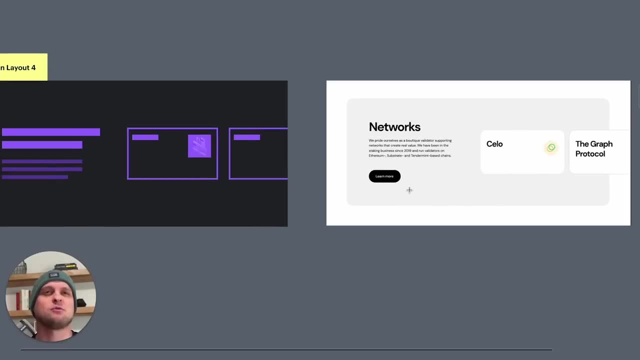 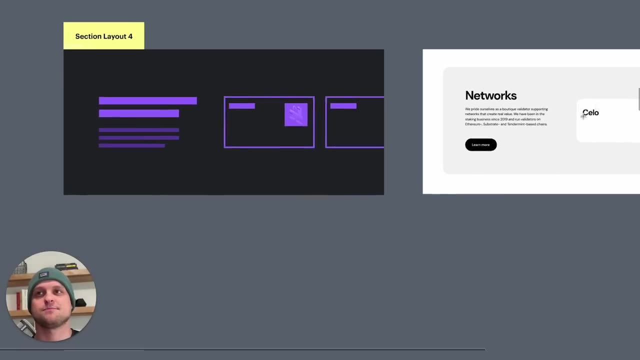 clickable arrow. So for this reason, I sometimes try to avoid sliders if at all possible, but this is a really cool way to incorporate a lot of content in a very small section. All right, so moving down to section layout five, this one is a little bit out there, And this is something. 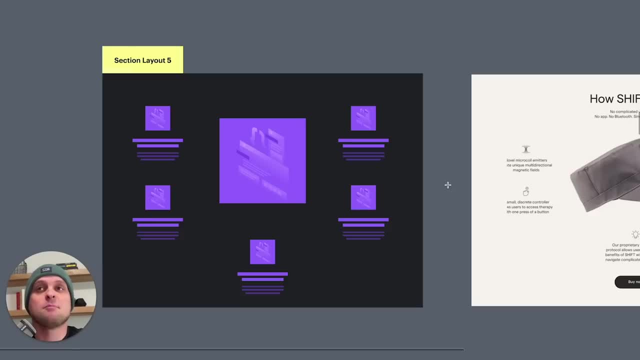 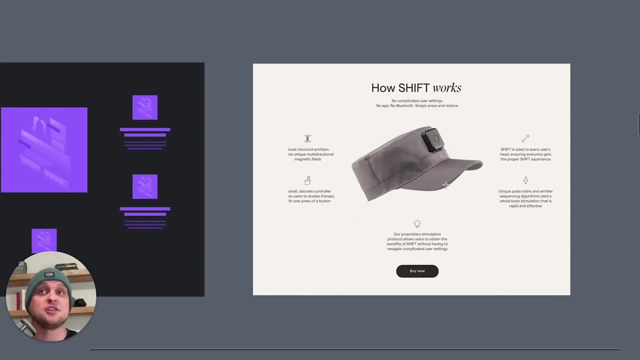 that I probably would not use on every single website that I've ever used. So I'm going to build, but I do love how well this works. in the example here with a product, They've got a product image in the middle and then they have all of these different icons and subtext all around the 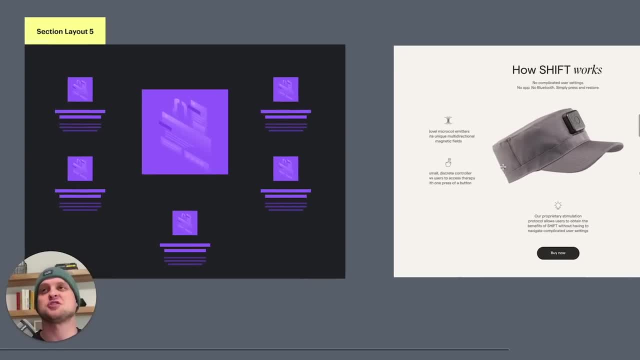 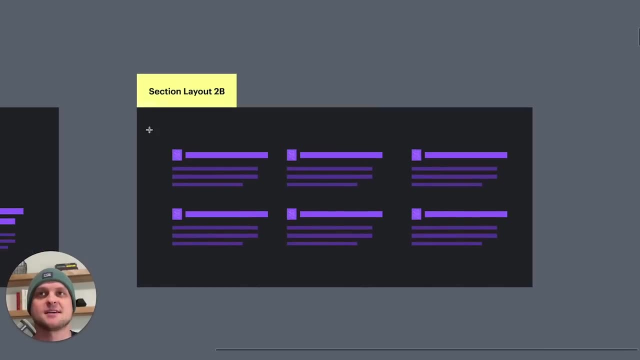 product. Now, the thing that's cool about this is they could have easily just used our section up here right with the multiple columns, and they could have had the icons, the header, the subtext and then maybe a big image of the product up above. But I do love that they got a little bit. 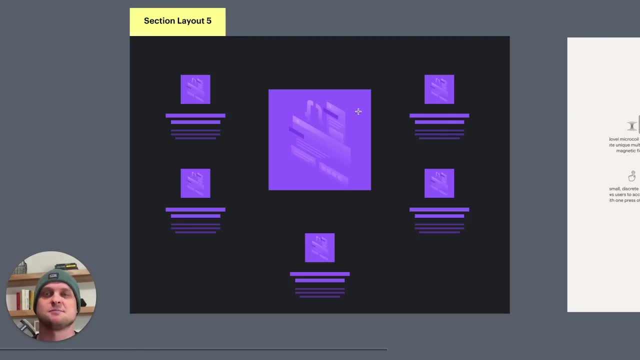 here and it just makes it feel like more of an experience, And it does make it feel like a very custom website, And so doing things like this might seem overwhelming because all of a sudden you're losing a lot of that control in terms of alignment right. It doesn't really feel. 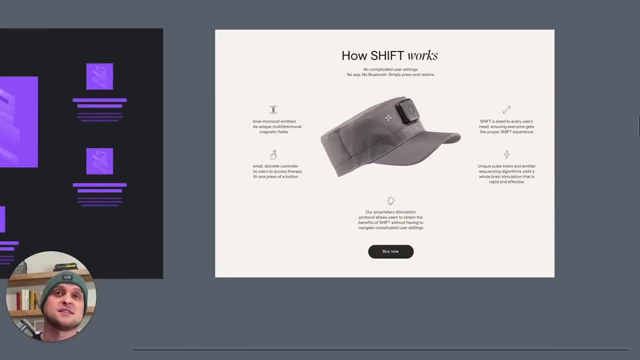 like things are very aligned, but if you really broke this down, you would be able to align these things pretty well. You can see here that basically they're just three columns and you can function with things that way rather than having to set position to. you know absolutely. 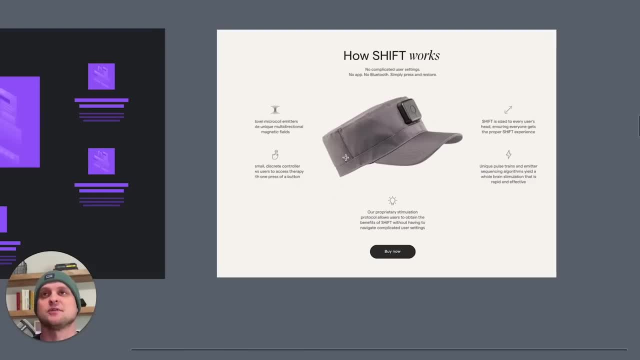 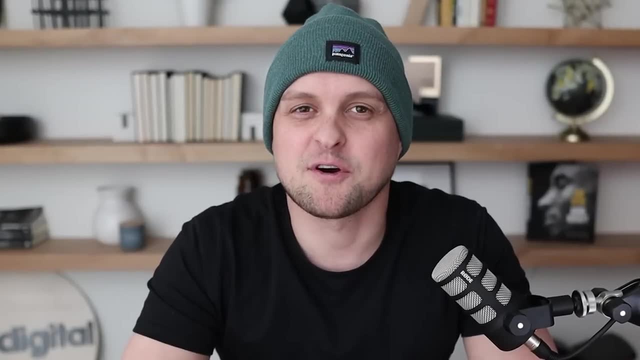 execute or whatever and move it around the page, And so this is a really nice layout. If you have, maybe, a product image and a lot of different bullet points, Hey, if you're liking this video so far and you want me to make another one just like this, with all new section last, that you've never 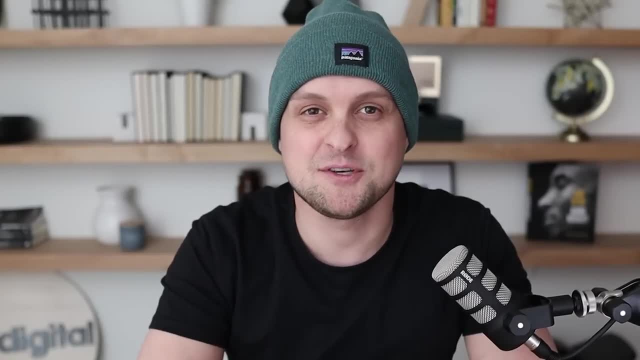 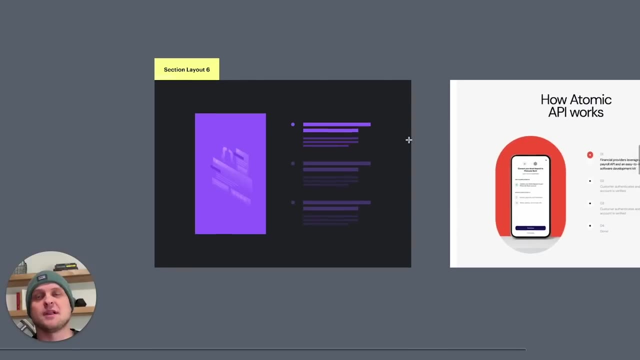 seen before. hit that like button down below, And if we get enough I'll be sure to make another one just like this. All right, let's jump back into it. All right. So, moving down to section layout six, I really do like this one And I think this is kind of a newer, fresher way to 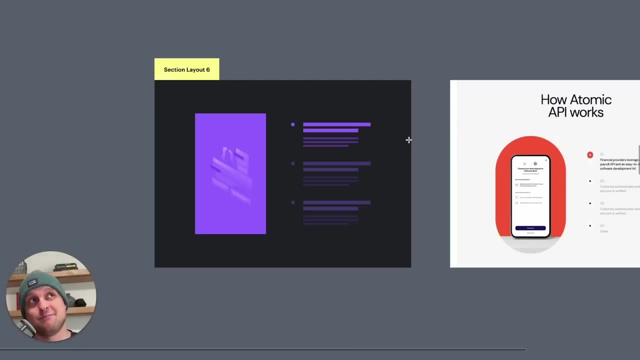 display a lot of content, especially if you have great images or, even better, if you have videos, And so what we've got here is we've got our asset on the left, and then we've got over here three bullet points, And you can see that the two below have an opacity set, showing that this one on 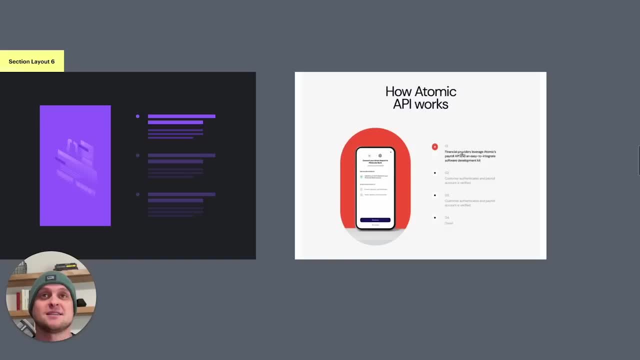 the top is the one that's active And our example over here. you can see that not only does it have this text darker, but also, as the bullet point, highlighted in their brand color, And so, essentially, what's going to happen with this is either it's set on a timer or 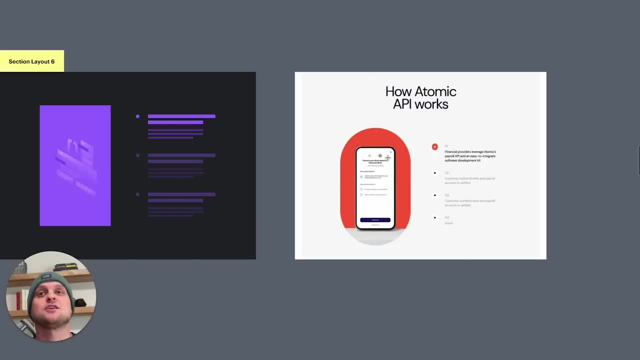 your, And so essentially, what's going to happen with this is either it's set on a timer or your or your clicking through, and every new bullet that you click it's going to change the image. Now I do see a lot of times where people are able to bring in really cool interactions. 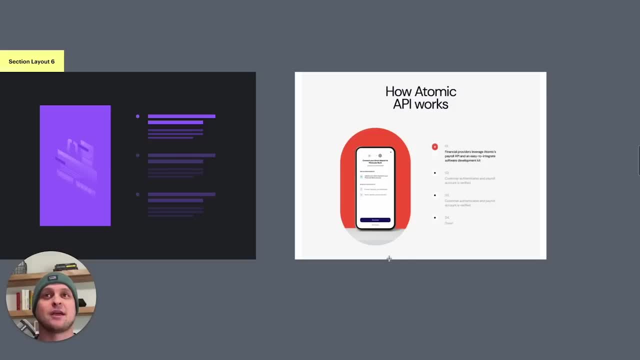 where, when you click, not only does it just change the entire image, but it would basically keep this red circle and the phone would slide out one side of the circle and the next phone or image would slide into the circle, And so this is a really cool way just to keep people 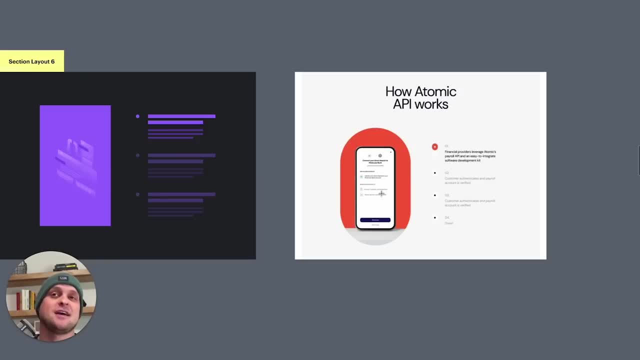 on one slider, but also keep them engaged and show them a lot of different images and information. Now, one thing that I would recommend is, if you're going to set something like this on a timer, there should be some sort of indicator showing them that it's working through it, And 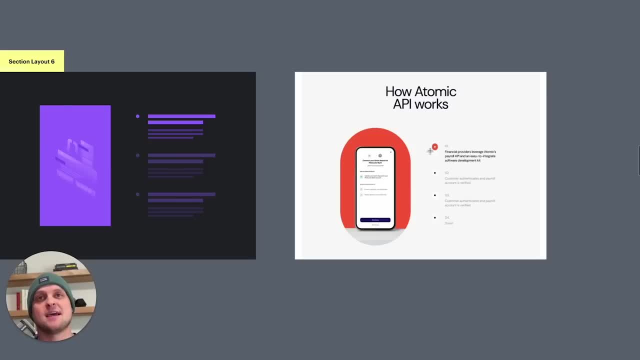 then it's going to hit the next step. And so in this example, even though this is a static image, I would hope that if this was set to say five seconds, and then it would turn to step number two, it would have maybe a reddish orange line, that kind of starts, to come down, And then when 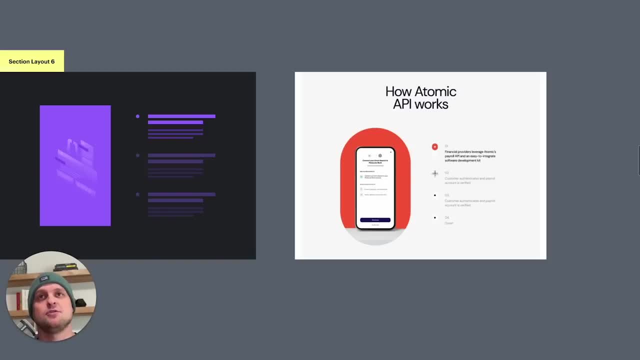 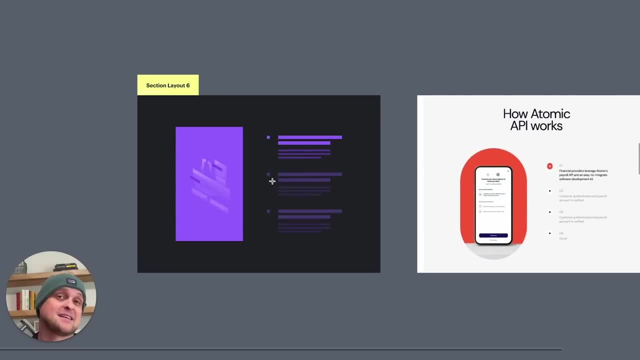 it hits the second bullet point. it then moves to step two and changes the image. So this is something as well that you could have left right aligned or right left aligned, It doesn't really matter, And technically you could do this vertically as a regular kind of tab slider. But 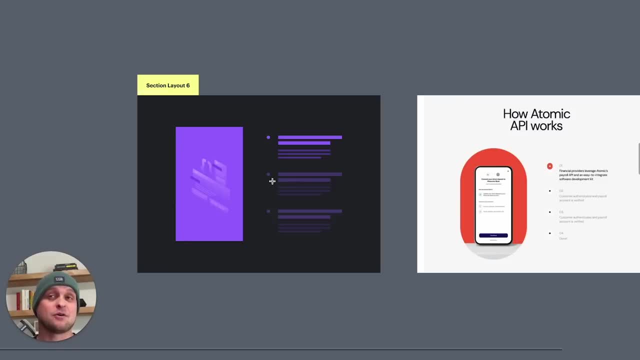 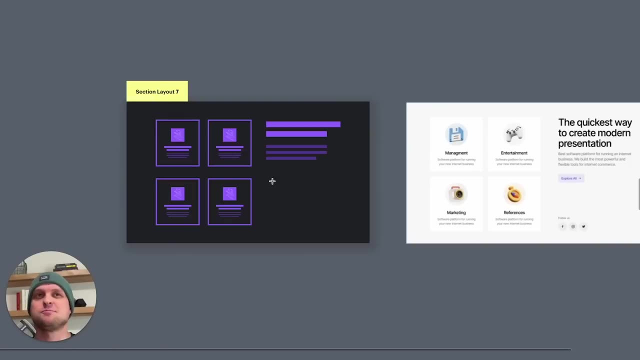 at the end of the day, this is a really cool way to lay out your information, especially if you have great images to share. All right. section layout number seven: this is basically just taking a kind of a two column right left align, And then within one of the columns you're adding a. 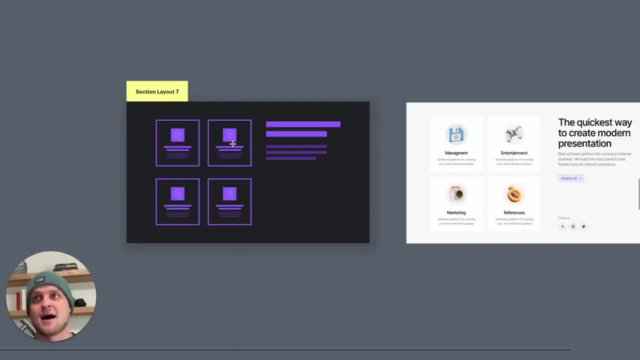 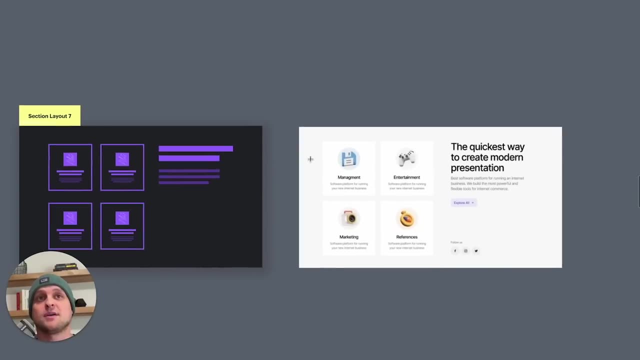 two by two grid, And within those then you have vertical right aligned icons, And so you're basically just taking a variation of a couple different layouts and squishing them into one. Now here's a really cool example You can see here that they've used. 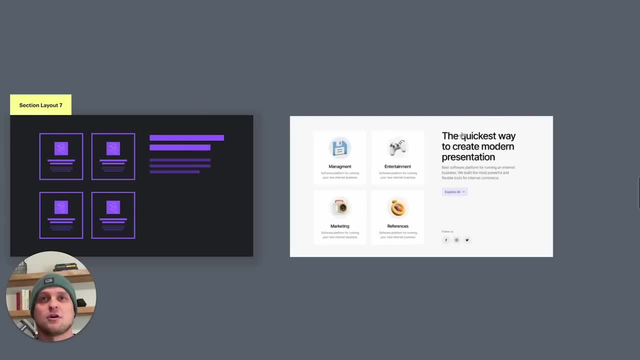 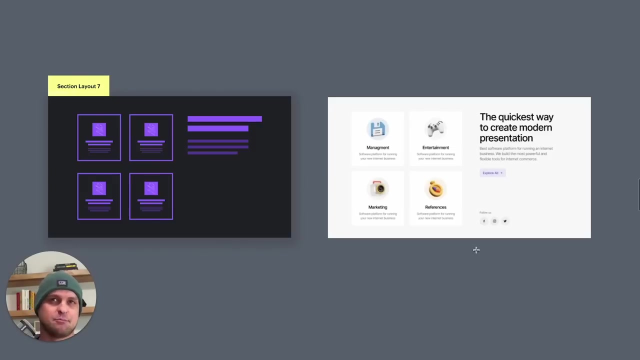 really cool, like 3d icons, and then they've got their content over here on the right And then down below they have their social media icons. Now, the thing that I do love about this is this just shows how easily you can bring together multiple different section layouts and templates. 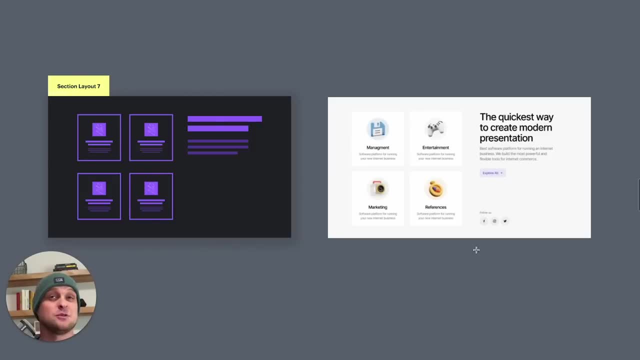 and basically just do Whatever you want with them. Another thing that I do like about this is we are oftentimes a little bit hesitant to put our content over on the right, And this is another thing that I would do very sparingly because, you know, as humans, we read left to right, And so typically, this is where our 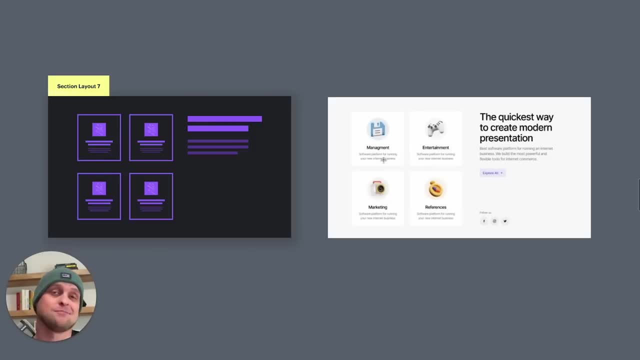 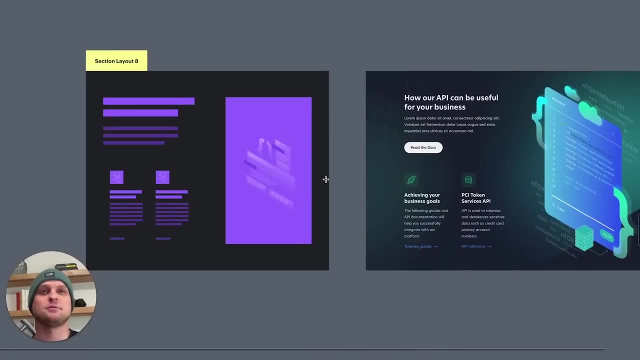 eyes are going to go first, but if you have some really good bullet points to share up here, it may not be a bad idea. All right, So going down to layout number eight, this is probably my favorite out of all of our layouts that we have in this. 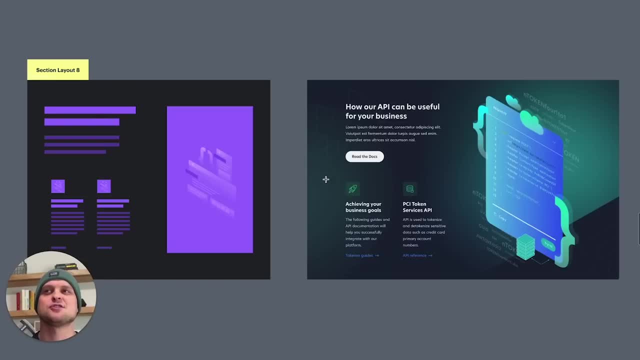 Okay. The reason is it's basic, but it just looks really, really clean. This is something that we see on a lot of websites, especially like tech websites like this example, that have really cool illustrations, They have icons, They have a lot of information. Websites like stripes website does. 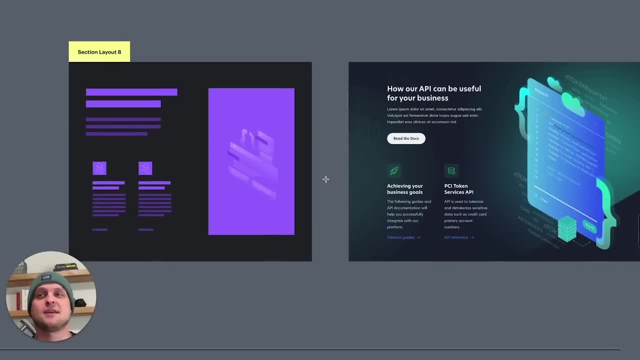 a really good job of this, but essentially what they're doing is they are just getting a combination of vertical and horizontal alignment and then just nesting it inside each other, And so if you look at this at its biggest element, this is your, your scroll line. this is kind of mix. You sort of go to it head text Run just. 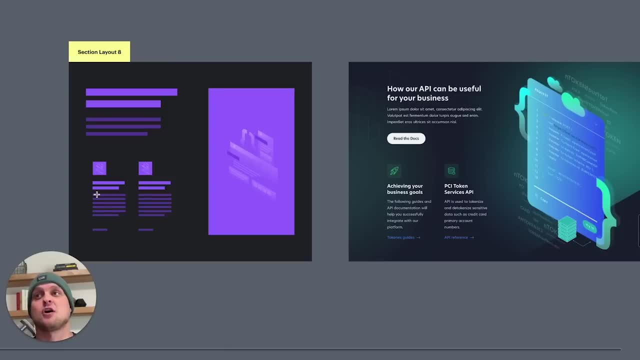 a play And it's exactly like this: You have a vertical line, you do a horizontal, you're a vertical, vertical and a horizontal and that sort of thing with that kind of look of it, And then you kind of nesting. θαo suggests to it that I'm not going to have this go over this. 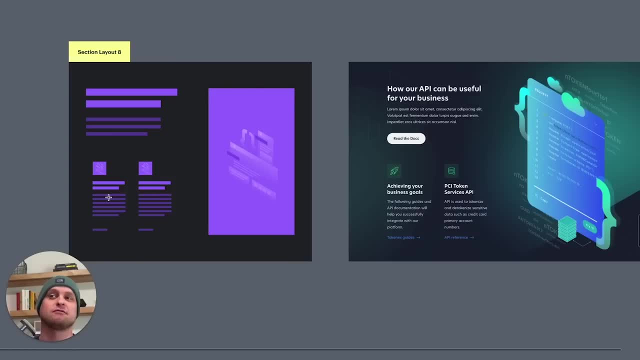 beginning line, go over this end point, do this work, go back up source, go to command, go to itemsgif. and I'm just going to go back to red Press and I'm going to just east press, right, Because you know you always end up getting a little more context going into that area, Like this: 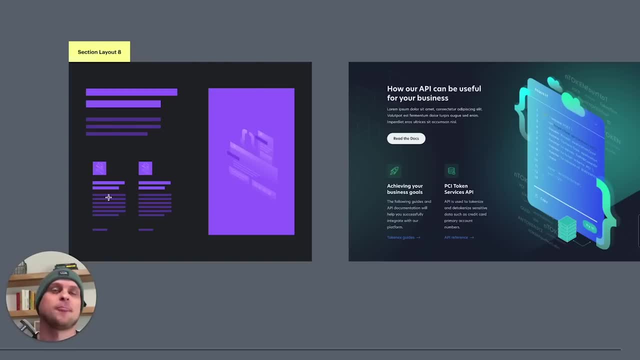 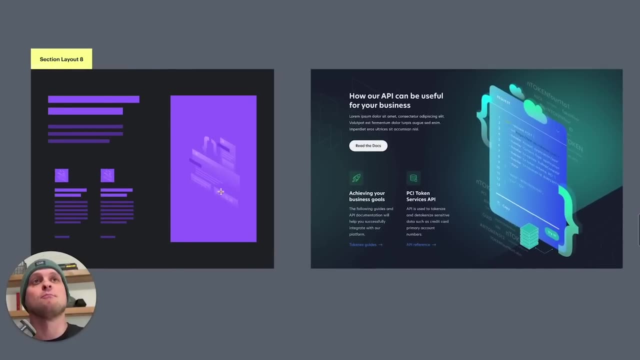 is just a two column Right. You've got your column here on the left with information and your column line. you can make this vertical whatever you need to do. But one thing that you're going to see a lot in different section designs is the more variation you can have between vertical and 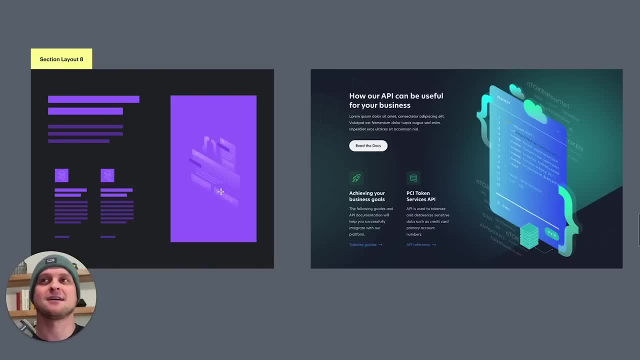 horizontal layouts, the more complex and custom it's going to look So. a lot of times on template websites we just see that standard two column horizontal layout. right, But if we can start to incorporate different images, icons, text blocks and then again going from horizontal to vertical, 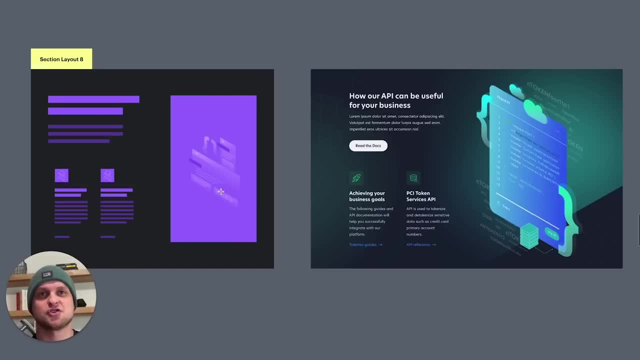 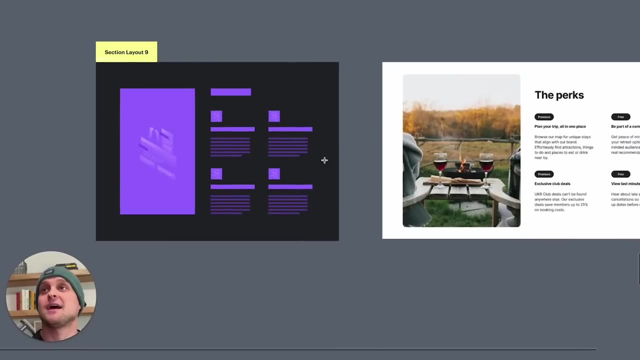 to horizontal, to vertical. it just makes it feel so much more custom, And so any chance that you have to do that, definitely take advantage of that. All right. So, going down to layout number nine, this is another great example of what we just talked about. You've got the image on the. 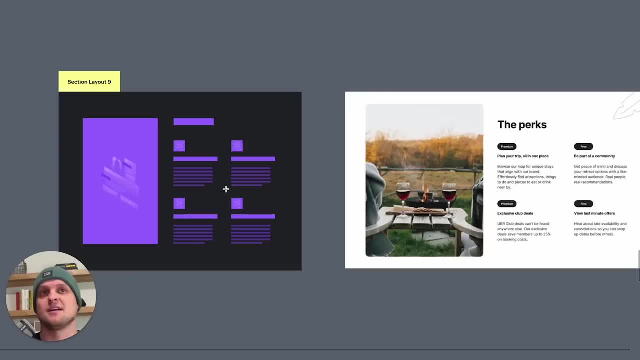 left and then on the right, we've got a four column layout. This is again another great way to kind of utilize your need to maybe highlight two, three, four, five, six different bullet points And instead of just putting them in, 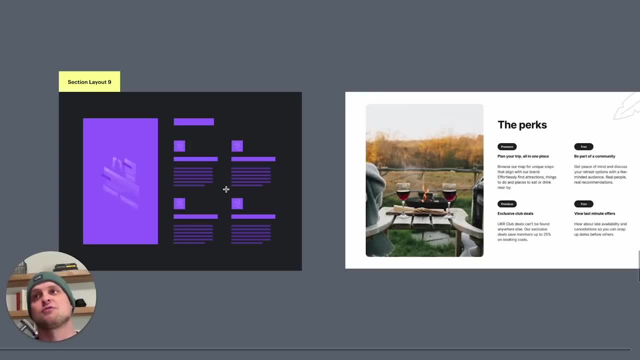 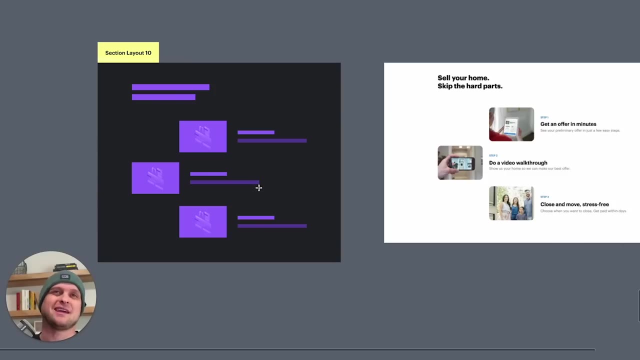 bullets or a very basic column layout. you can throw an image on the left, add a header up top And then again we're just nesting horizontal vertical, horizontal, vertical and giving it a really complex feel. Section layout number 10.. This one is a little bit more unique And I 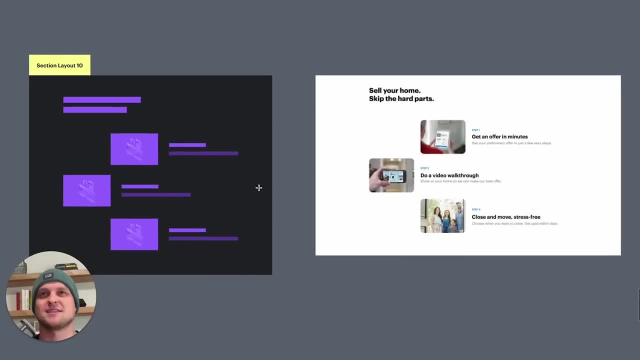 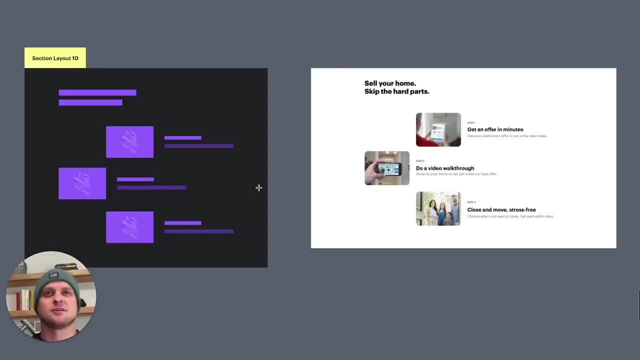 actually really like this At first. when I look at it it makes me a little bit uncomfortable because it feels like nothing is really aligned. But the more you look at it you'll see that it's really well. They just have given it a little bit more flow, And it is while it might be. 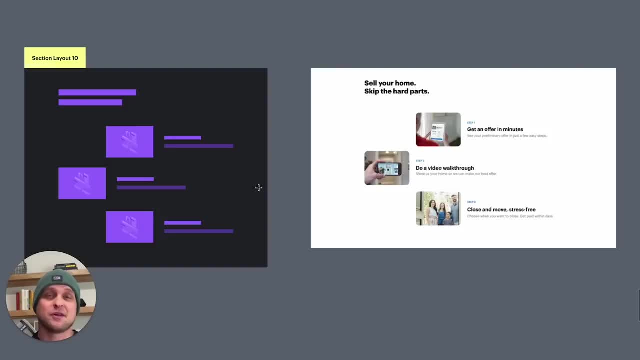 uncomfortable to look at. design wise, I think it's done pretty well and it is engaging, And so you can see here that if we had things left aligned, we've got our header and then our second bullet is aligned here, And then our first and third images are aligned with the text here, And so 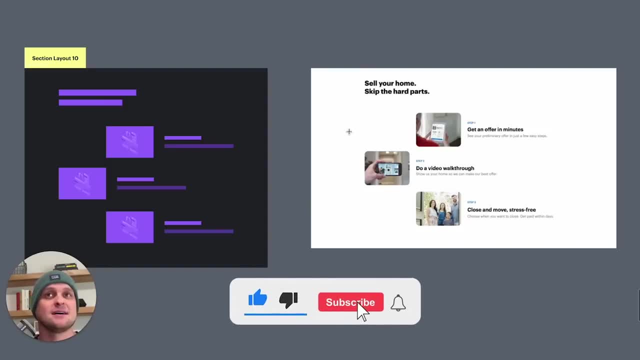 basically what they've done is they've just add some space or padding to the first and third one, just to slide them over, And it does just kind of feel like it takes you back and forth as you go through the steps. So again, this is another unique way to approach this problem of just having these 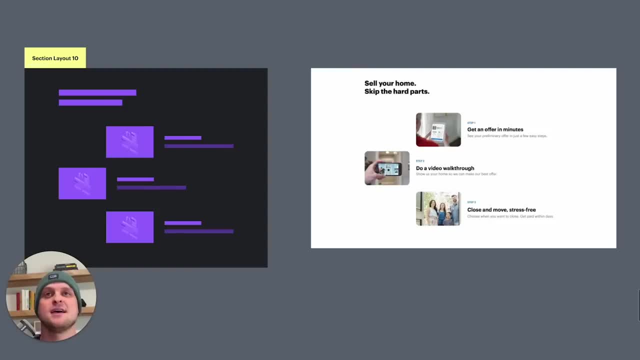 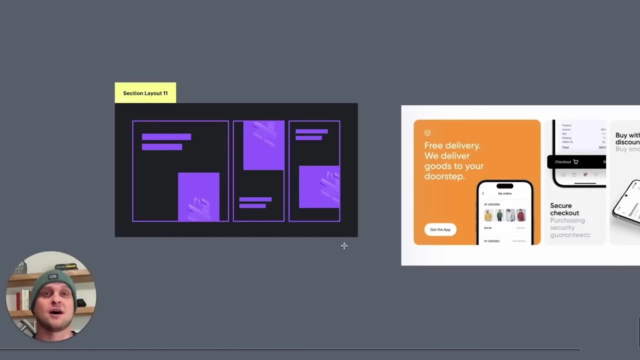 three bullet points with three images or three icons, And it's going to be really, really useful for you to look for different ways to display this other than always defaulting to just that three column. look. And finally, our section layout 11.. This one is done a lot, especially recently. I 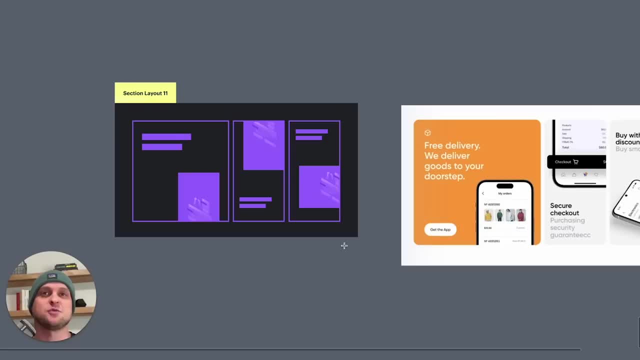 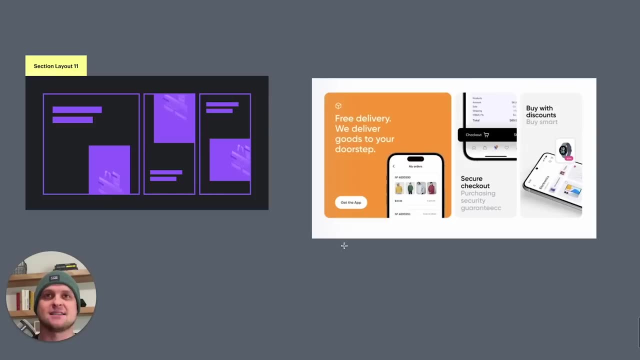 feel like there are a lot of great companies that are doing this And essentially, what they're using is just a grid and they are just resizing and making each different grid element a different size, And then you can show priority, of which one is most important, of course, by putting on the 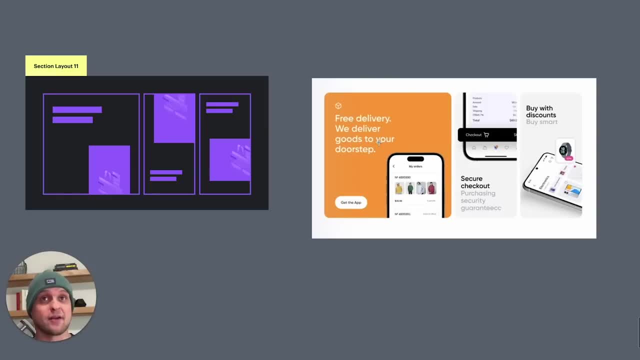 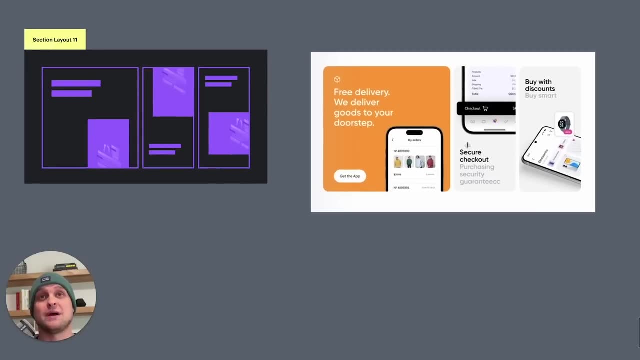 left, maybe adding color and then making it the largest grid area, But also it just gives you a lot of different ways to lay things out, And you could continue this layout all the way down, and maybe right below this you flip it, or maybe the center one becomes the center one, And then you 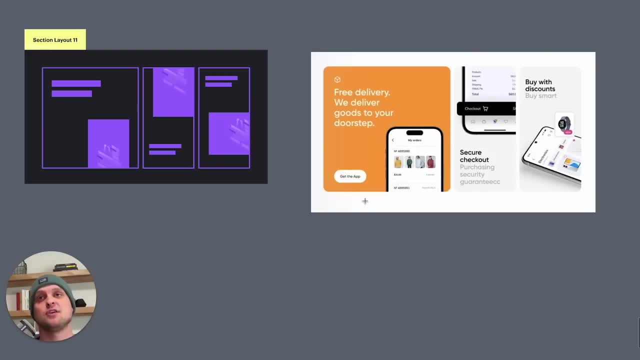 can see that this is the largest, But using this type of grid and then just putting your images and text inside of div elements, this is a really cool way to just be unique while also having your layouts be about as simplistic as you can, And so I'll show some examples here of companies that 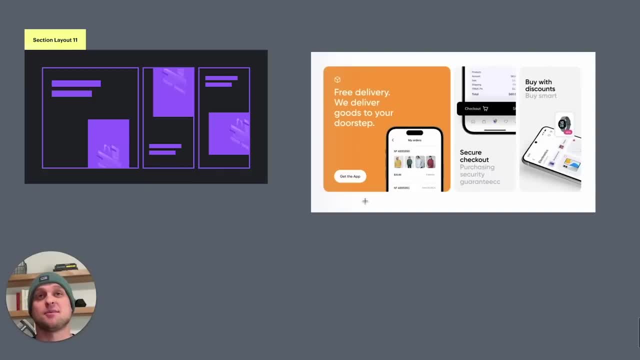 are doing this, but I really do like this layout And this is something that I need to push myself to incorporate more into my designs, because sometimes it feels like it's too basic and too much like a template, And once you do it right, you're going to be able to do a lot of different. 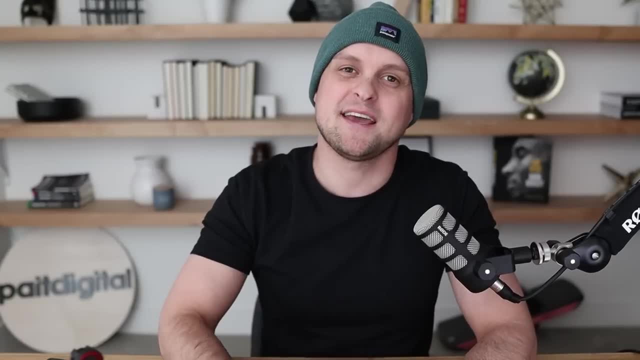 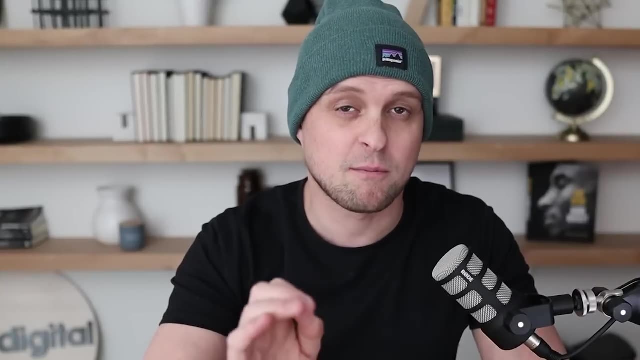 things. It actually looks really good, All right, So I hope that you can take all of these layouts that we covered today and start implementing them into your websites. It's going to improve your work so much. Now, if you want to learn more ways on how to make your 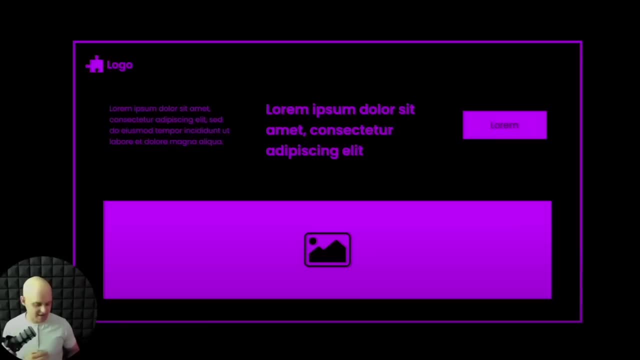 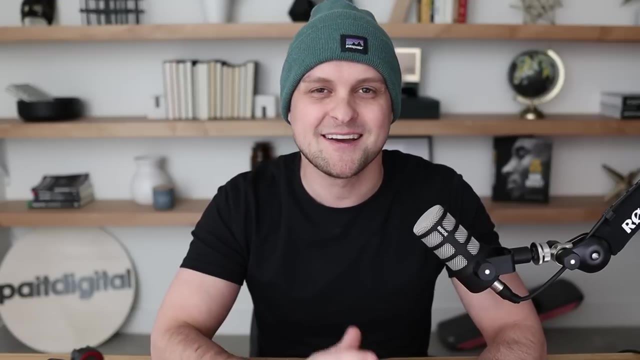 websites feel custom and unique. I recently posted a video on a ton of different variations of hero section designs that you don't want to miss, So you can click that video up here in the top corner. I hope you enjoy it. Thanks for watching and we'll catch you in the next video.